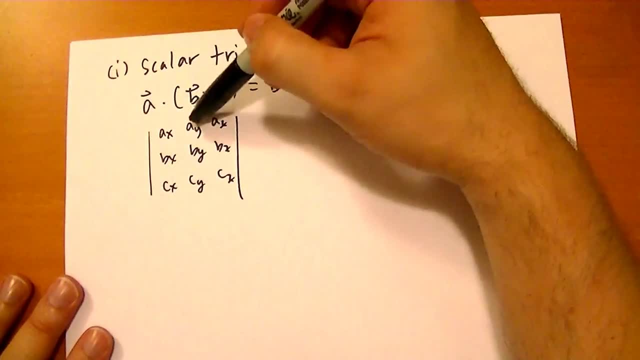 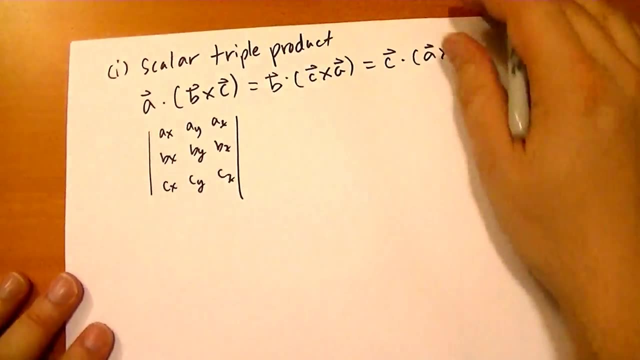 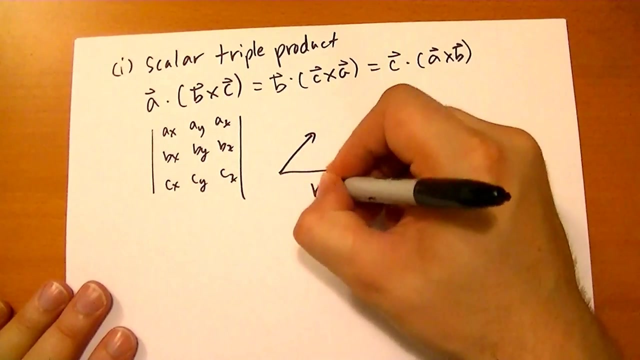 the I hat term is going to be multiplied by the ax, and the coefficients of the J term is going to multiply by a Y and the coefficients of the Z term are going to multiply by AZ. so it works out. it's great. the geometric interpretation is suppose you had three vectors- C vector, cross B vector, and this is actually the. 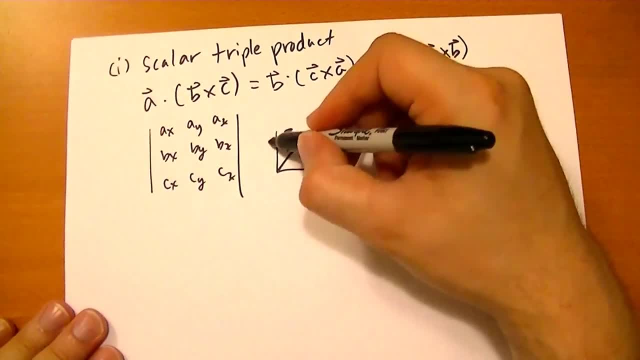 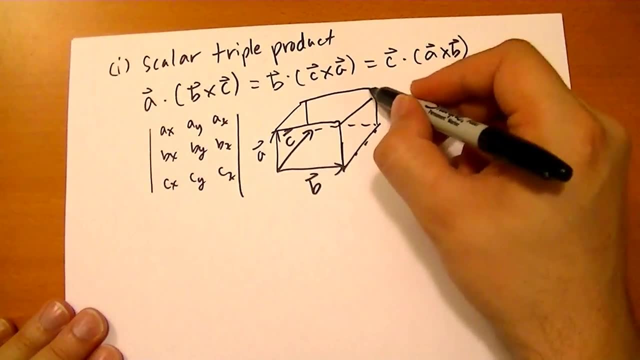 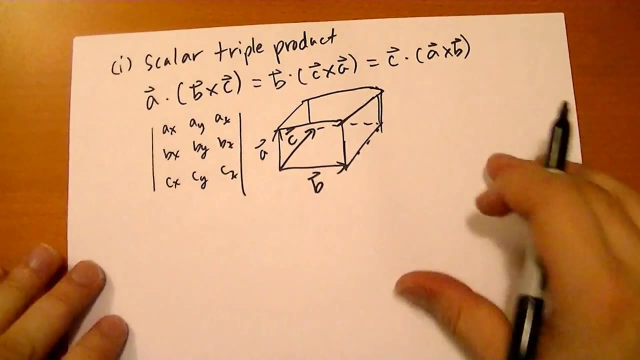 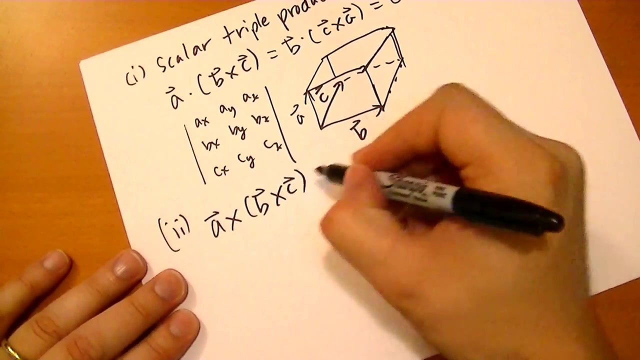 area of that parallelogram. and then if we had an, a vector to boot, then what we would get is the volume of the parallel pipe head defined with a corner like that. so rather simple. the second triple product that's interesting is the triple cross product, and that follows the back cab rule, so ba. 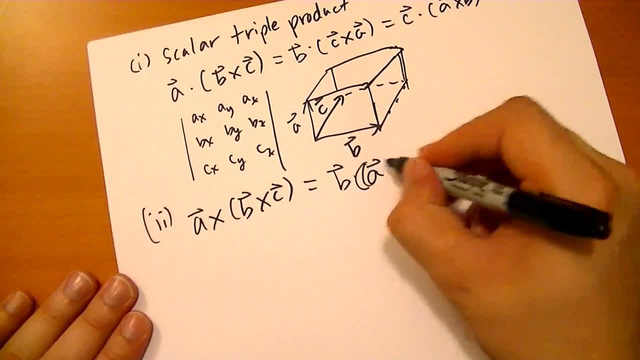 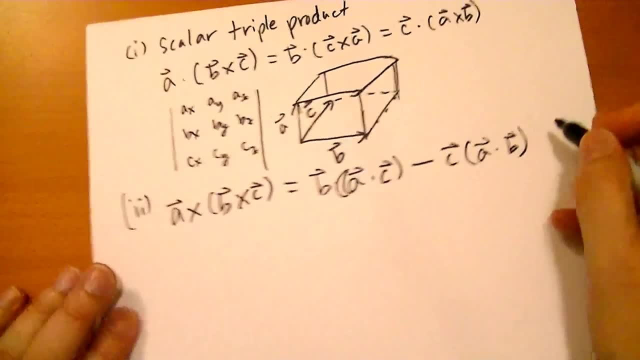 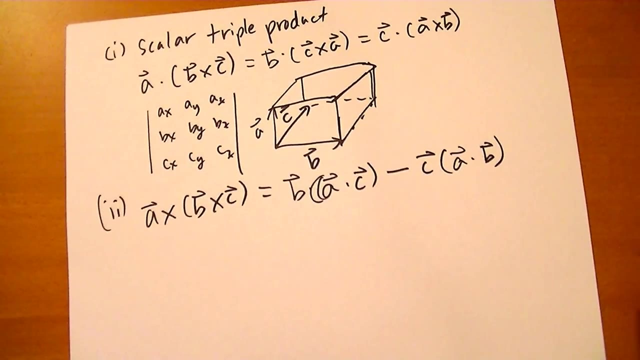 no, it's just B times the quantity a vector dot C vector, minus C vector times the quantity cab dot B vector. if you reverse the terms of this one, then obviously you're going to have a negative. so you have to switch the two terms, the back cab terms, incidentally, using these two rules, all higher triple cross. 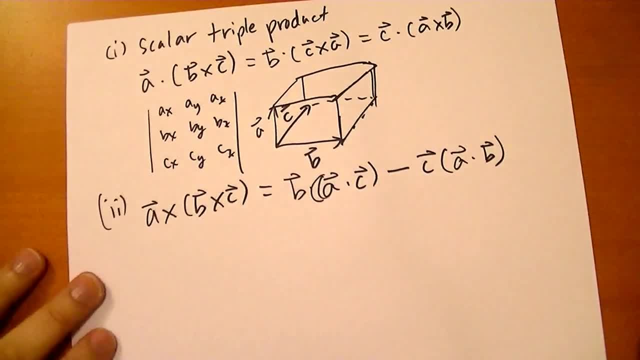 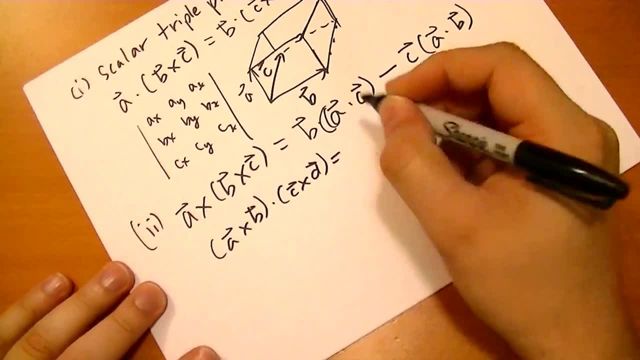 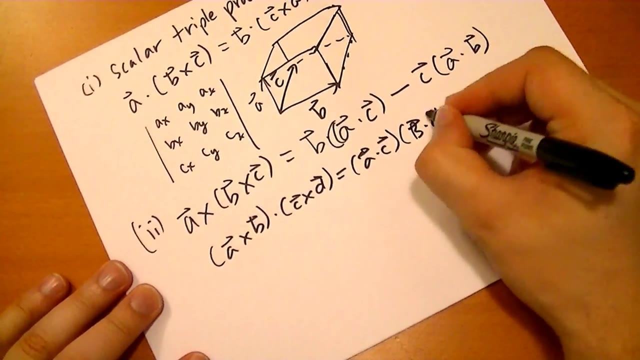 products can be derived. the two that they list in the book that are interesting are: A cross B dot C vector, cross D vector. and that turns out to be the same as a vector dot C vector times B vector, dot D vector minus a vector dot D vector B vector dot. 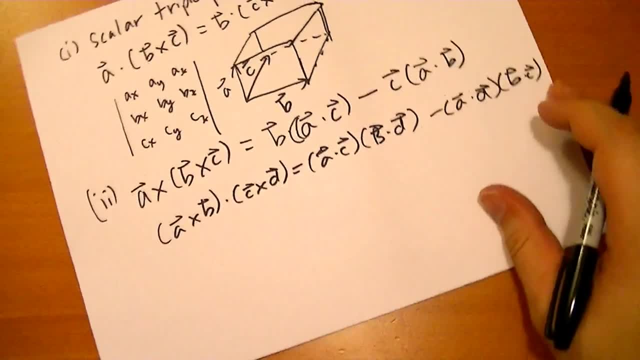 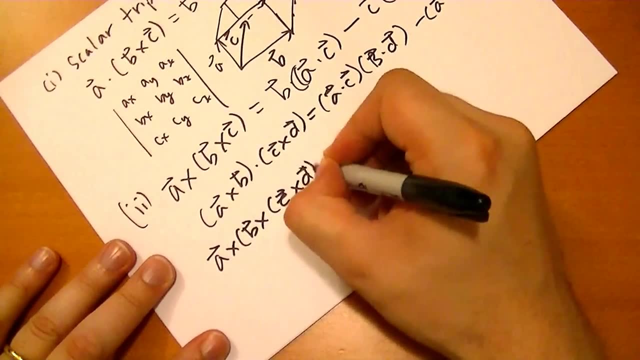 C vector and the other one they have, like if you're crossing one after the other. so you have a vector, cross B vector, cross C vector, cross D vector, and what happens? there? Is that too many parentheses, That is, Oh, let's put one here. 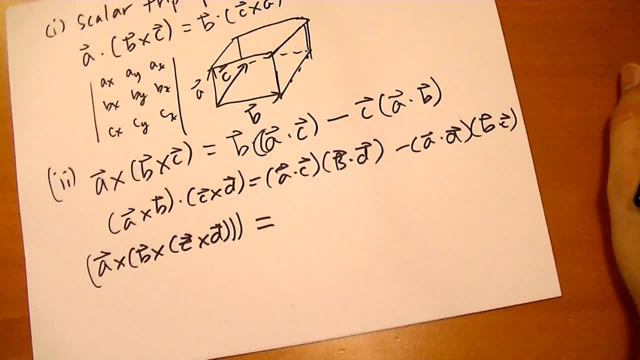 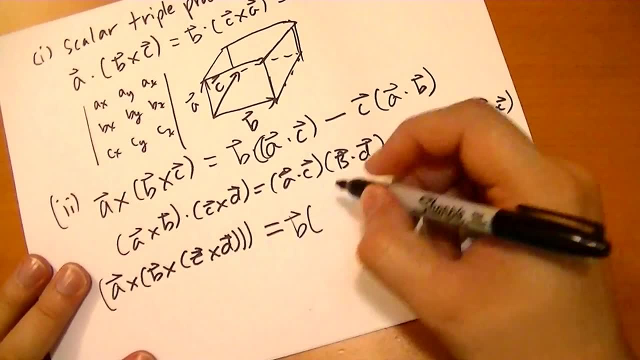 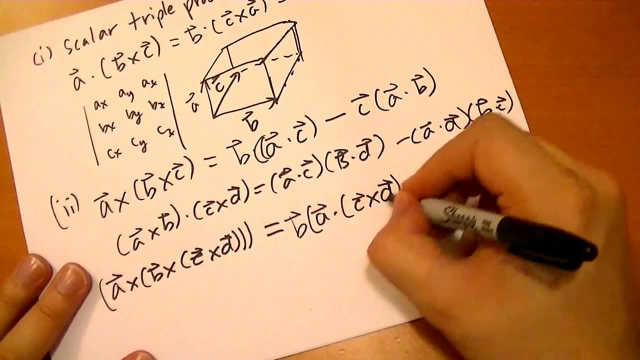 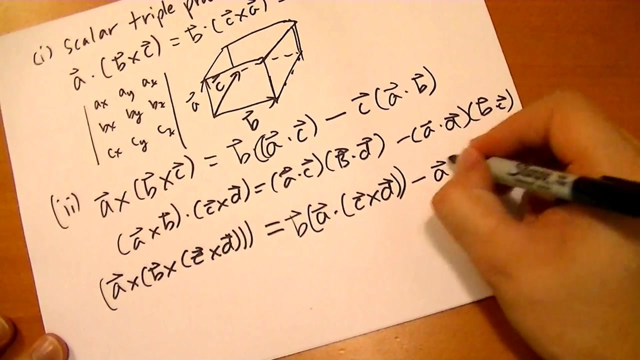 It could. even So it follows the bat-cab rule, except for that C vector is actually C cross D. So you go ba, That's the volume, That's the scalar triple product right there, And then the other terms can be simplified.